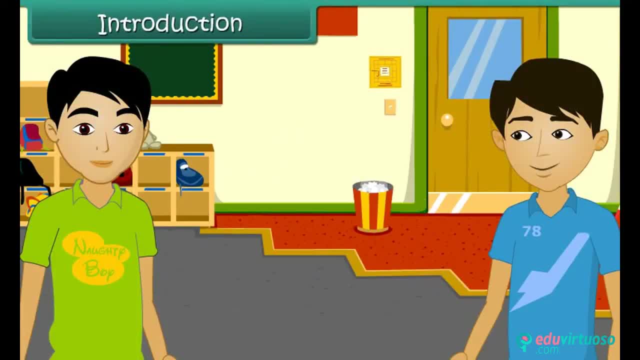 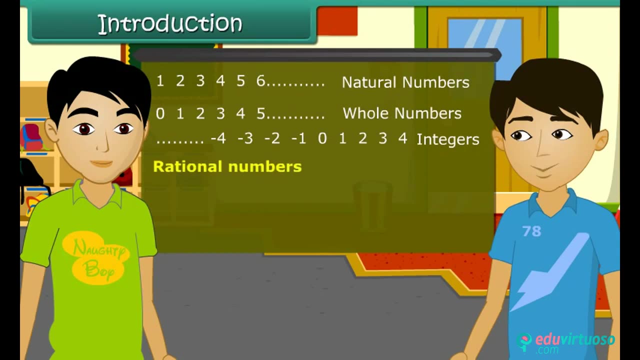 Introduction. What are you doing, Amit? Hey, Rahul, come You know. today, our maths teacher taught us a new topic: rational numbers. I know about natural numbers, whole numbers and integers, But what are the rational numbers? These numbers are in the form numerator by denominator. 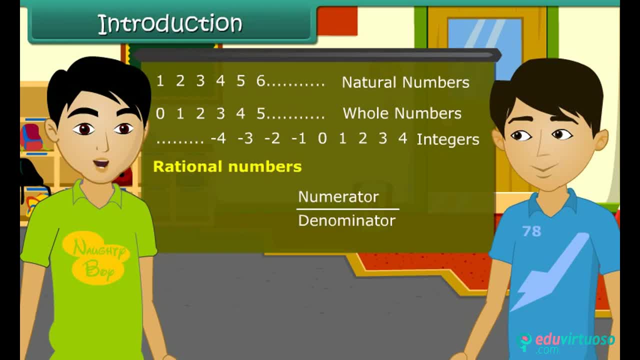 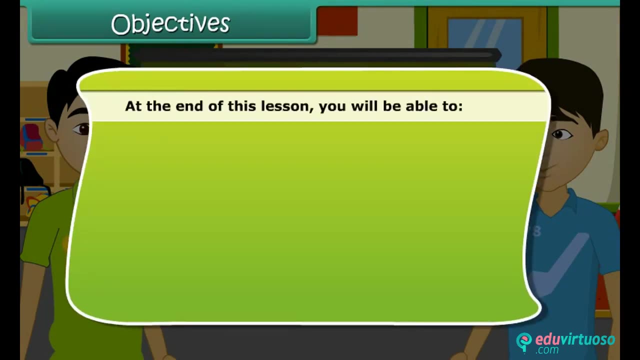 where numerator is either zero or a positive integer and the denominator a positive integer. I did not understand Come. I will explain you Objectives. At the end of this lesson, you will be able to define rational numbers, write equivalent rational numbers. 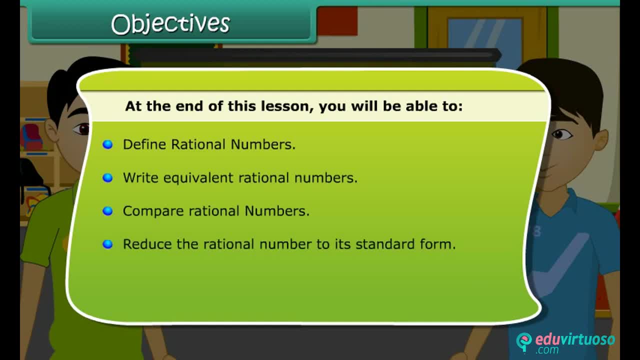 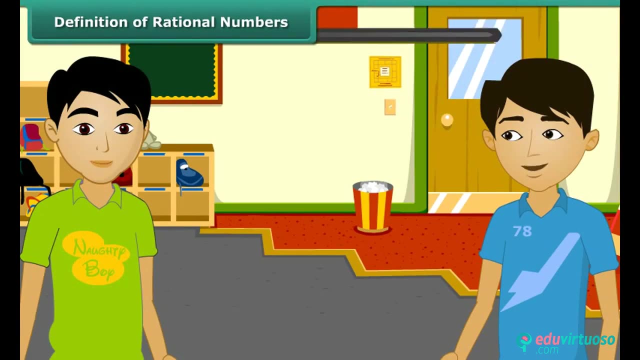 compare rational numbers, reduce the rational number to its standard form, add, subtract, multiply and divide rational numbers. The word rational is a word that means rational arises from the term ratio. You mean that a ratio like 3 to 2, which can also be written as: 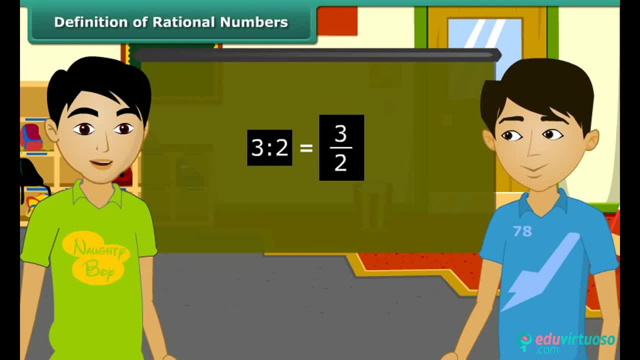 3 by 2 is a rational number. Yes, Similarly, the ratio of two integers, p and q, in which q is not equal to zero, can be written in the form b by q. This is the form in which rational numbers are expressed. 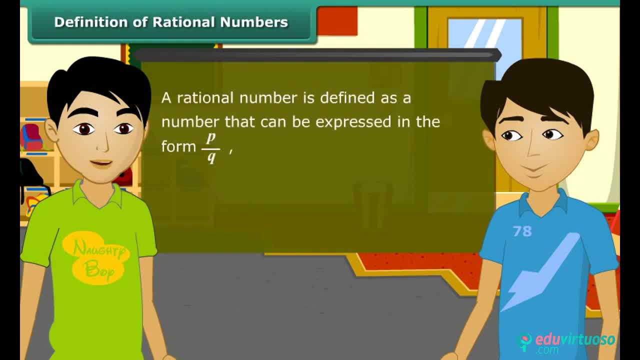 A rational number is defined as a number that can be expressed in the form P by Q, where P and Q are integers and Q is not equal to 0.. Rahul, now you tell, Is 4 by 5 a rational number? Yes, 4 by 5 is a rational number. 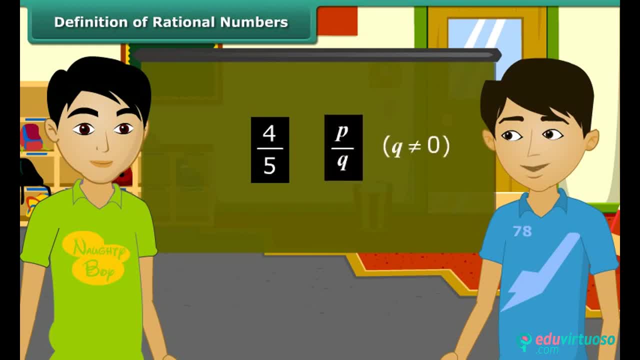 because it is in the form P by Q, where Q is not equal to 0. And is minus 3 by 4, also a rational number? Yes, because P is equal to minus 3 and Q is equal to 4 and both are integers. 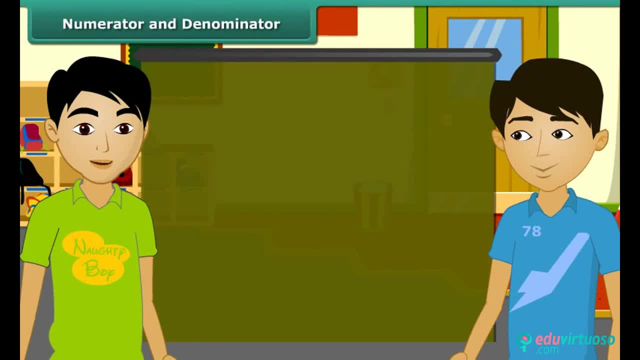 Do you know what is numerator and what is denominator? In rational number P by Q, P is a numerator and Q is a denominator. For example, in minus 3 by 7, the numerator is minus 3 and the denominator is 7.. Amit, are integers also rational numbers? 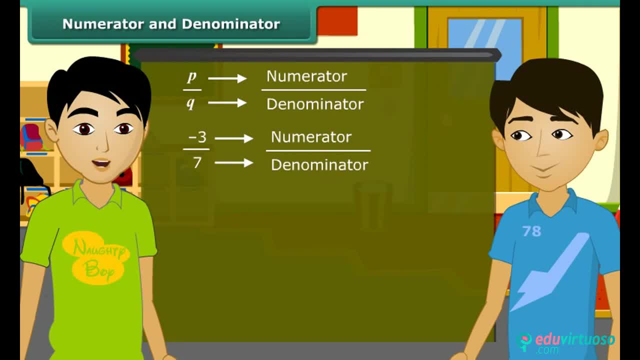 Yes, for example, the integer minus 5 is a rational number because you can write it as minus 5 by 1.. Similarly, the integer 0 is a rational number, because 0 can also be written as 0 by 2 or 0 by 7, etc. 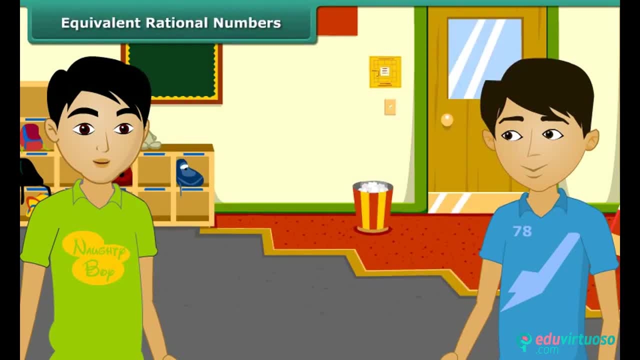 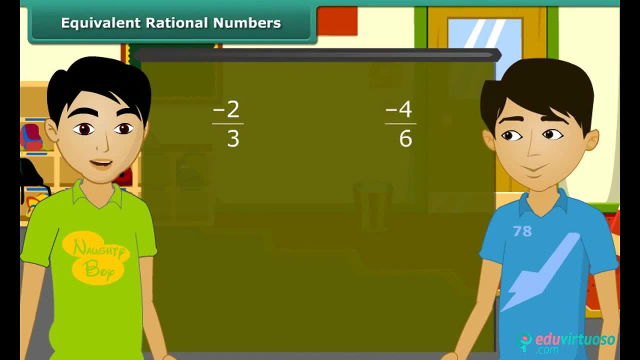 I will now tell you about equivalent rational numbers. Look at this rational number. Now look at this rational number. These both rational numbers are equivalent. But how? When? we will multiply the numerator and denominator of a rational number by the same non-zero integer. 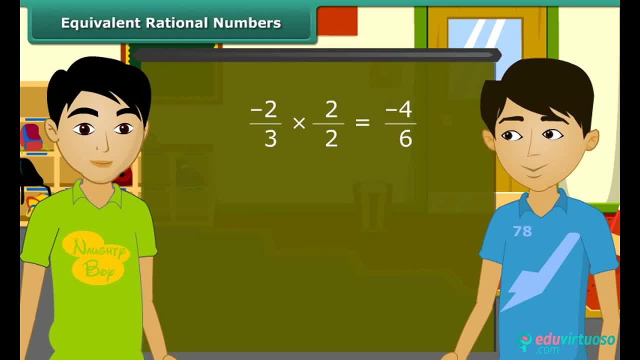 we obtain another rational number which is equivalent to that number. Similarly, minus 2 by 3 is equivalent to minus 10 by 15, because when we multiply the numerator and denominator by 5, we get minus 10 by 15.. Do you know what do we call a rational number? 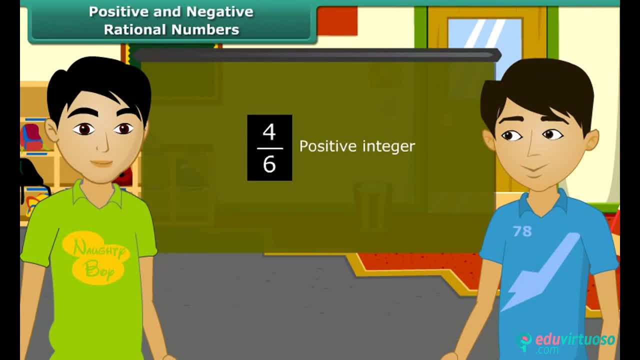 which has positive numerator and positive denominator. That rational number is called a positive rational number, I guess. And what are the negative rational numbers When the numerator is a negative integer and the denominator is a positive integer? for example, minus 4 by 7? 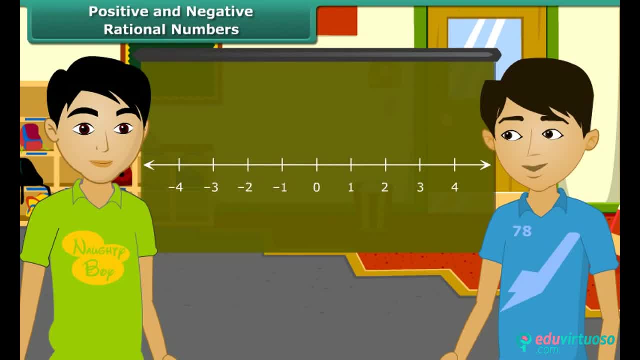 how do we represent a rational number on a number line? Look at this figure. This is a rational number line. Points on right side of 0 are called positive integers and points on the left side of 0 are called negative integers. Let's mark 1 by 2 on this line. 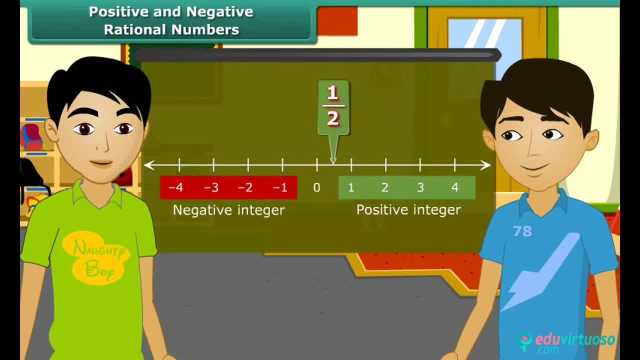 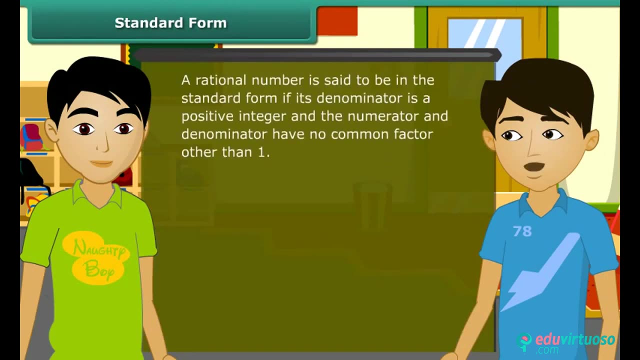 1 by 2 will lie in between 1 and 0.. And minus 1 by 2 will lie in between 0 and minus 1.. Now read this statement. Now read this statement. A rational number is said to be in the standard form. 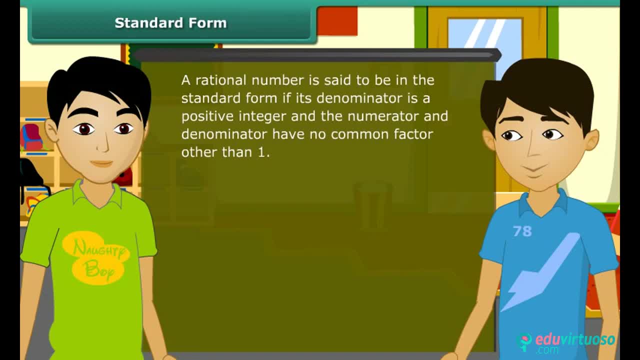 if its denominator is a positive integer and the numerator and denominator have no common factor other than 1.. That is, these all rational numbers are in the standard form? Yes, because their numerator and denominator have no common factor other than 1.. And if the numbers are not in the standard form, 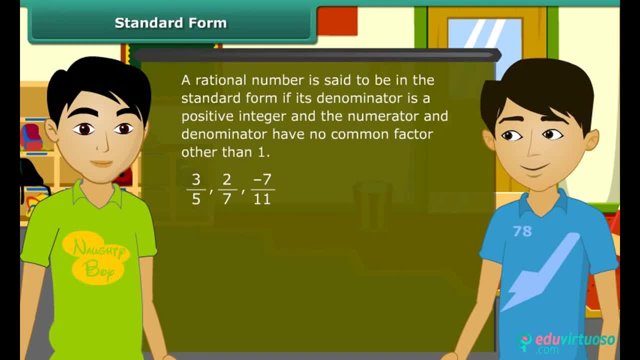 then it is reduced in a standard form. For example, minus 45 by 30 is not in a standard form. We will reduce it by dividing its numerator and denominator by their HCF. Here the HCF of 45 and 30 is 15.. 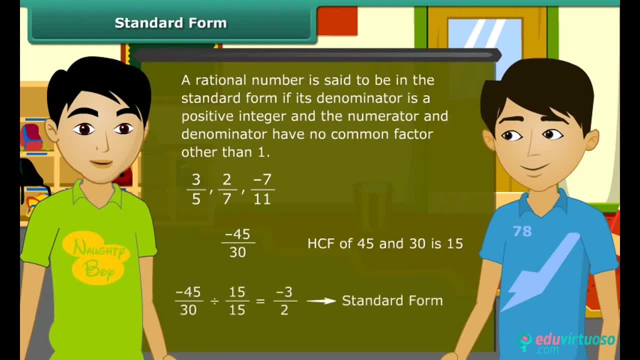 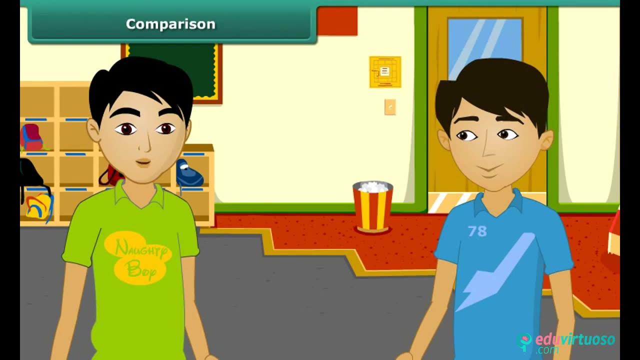 Yes, so we will divide the numerator and denominator by 15 and we will get the rational number minus 3 by 2, which is in a standard form. If we have given two rational numbers, then can you compare them? No, I will tell you how to compare rational numbers. 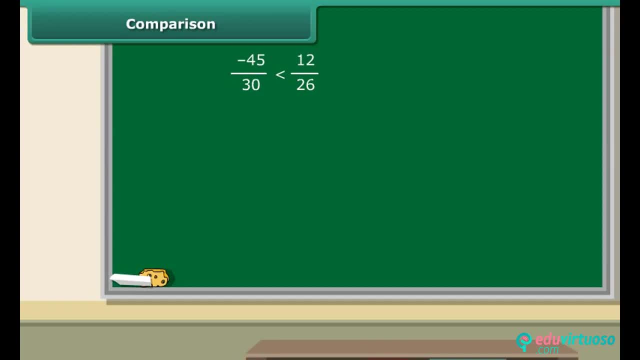 We know that the negative number is always smaller than the positive number. We can also compare the rational numbers using number line. The more the number is in the right, the greater it is. For example, 2 by 3 is equal to 1.. 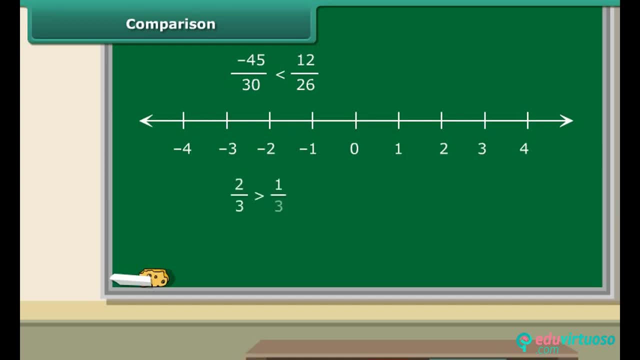 2 by 3 lies here and 1 by 3 lies here, So which one is in the right? 2 by 3.. Correct, Therefore, 2 by 3 is greater than 1 by 3.. Similarly, minus 1 by 3 is greater than minus 2 by 3. 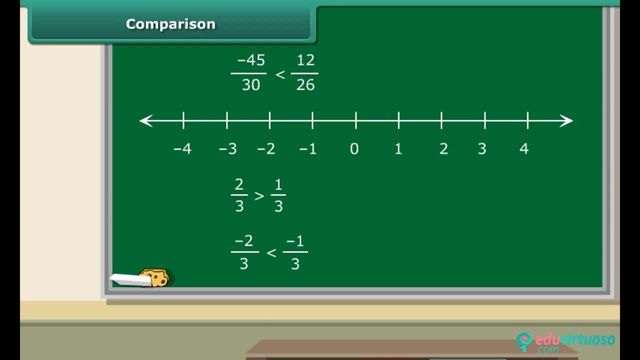 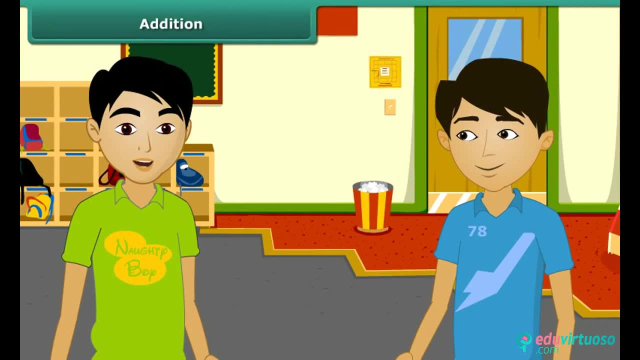 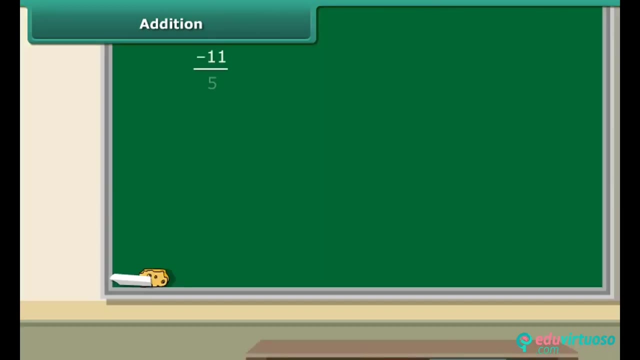 because minus 1 by 3 comes right to the minus 2 by 3.. Can we add the rational numbers? Yes, If the denominators of the rational numbers are same, then we just add the numerators. For example, minus 11 by 5 plus 7 by 5 is equal to minus 11 plus 7 by 5. 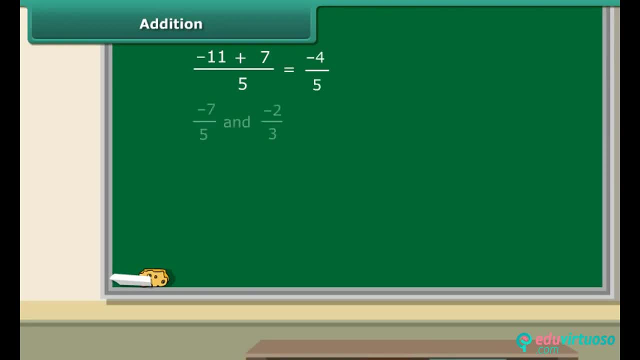 which is equal to minus 4 by 5.. And if the denominators of the rational numbers are not same? In that case, firstly we find the LCM of the denominators. Here the LCM is 15.. Then we find the equivalent rational numbers of the given rational numbers, 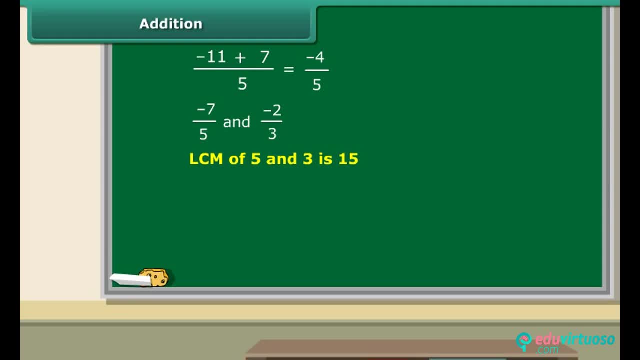 with this LCM as the denominator Here. minus 7 by 5 is equivalent to minus 21 by 15, and minus 2 by 3 is equivalent to minus 10 by 15.. Then add the two rational numbers Like addition when the denominators are same. 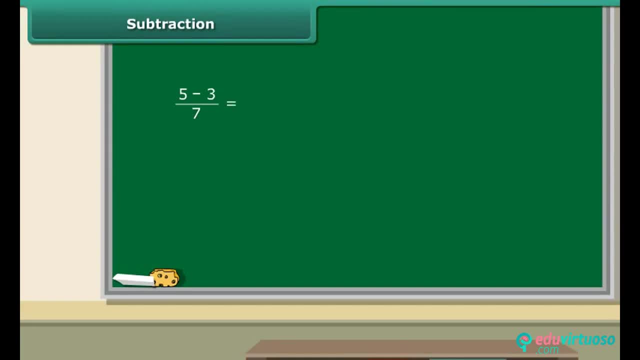 then we just subtract the numerators and keep the denominators same. And if the denominators are not same, we find the LCM of the denominators. Then we find the equivalent rational numbers of the given rational numbers, with this LCM as the denominator. 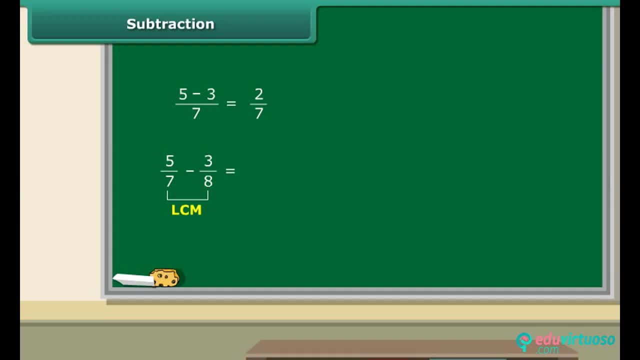 Then we find the equivalent rational numbers of the given rational numbers with this LCM as the denominator. Then subtract the two rational numbers. Can you guess how can we multiply rational numbers? While multiplying a rational number by a positive integer, we multiply the numerator by that integer. 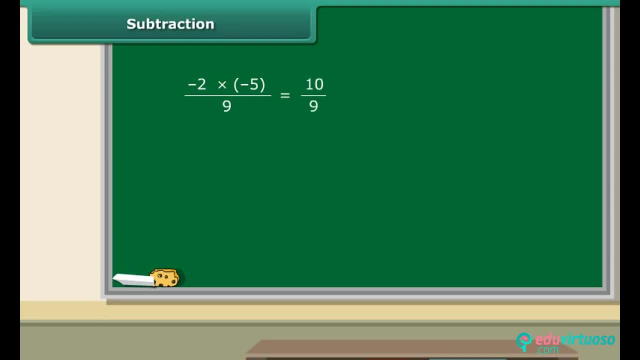 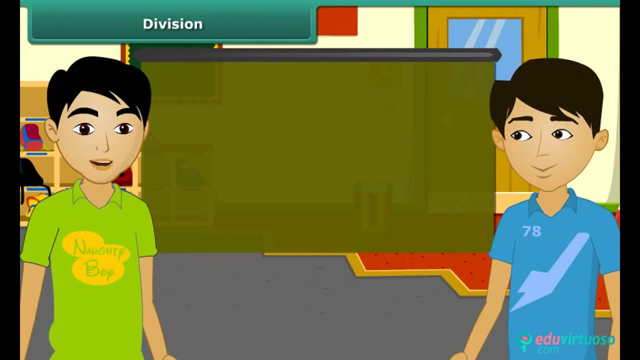 keeping the denominator unchanged. When we multiply the rational numbers, we multiply the numerators, then we multiply the denominators. Well done, You have learnt. now, Before starting about division, I will tell you about reciprocals. What are reciprocals? 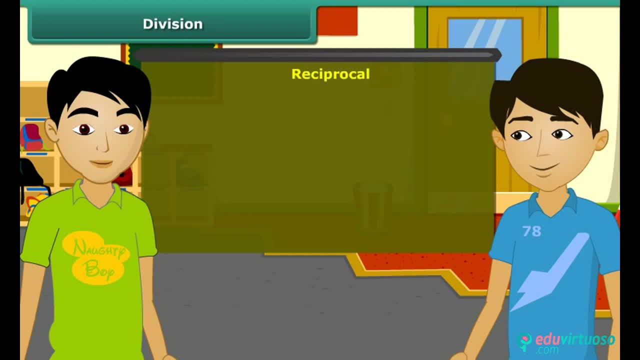 Let's take an example. The reciprocal of 2 by 7 is 7 by 2.. The reciprocal of 7 by 9 is 9 by 7.. Okay, okay, I got it. The reciprocal of minus 5 by 4. 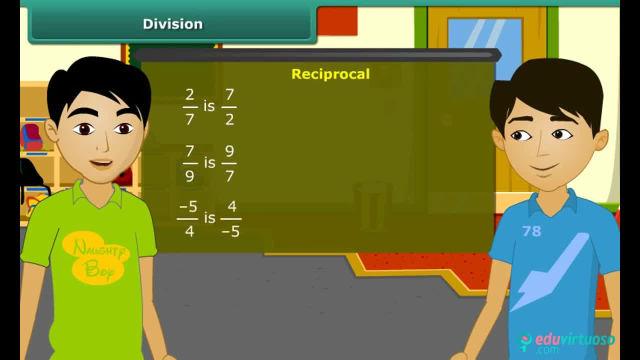 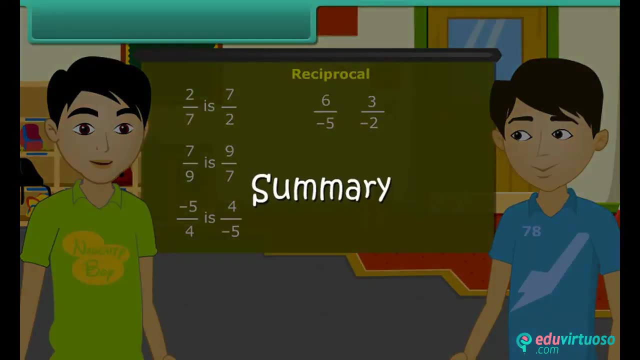 is 4 by minus 5.. Correct. So when we divide one rational number by another rational number, we multiply the rational number with the reciprocal of the other number. Summary- Let us summarize what we have learnt. A number that can be expressed in the form.